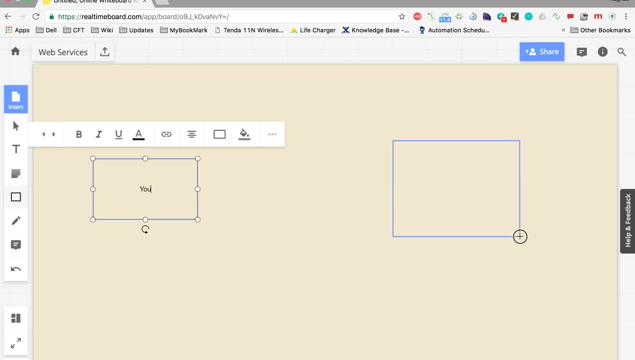 this is you, and let us say: this is the kitchen from where the food will be served. So let us say: this is the kitchen. Okay, now, what we are going to have is we are going to communicate our order to the kitchen and the kitchen is going to serve our order. Okay, now there. 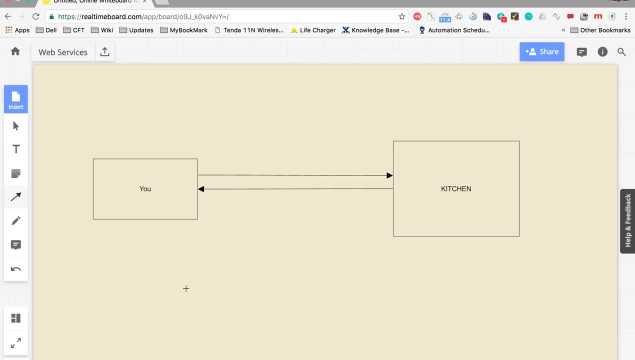 is an, a person who is involved in this communication process. The person takes your order from your table, goes to the kitchen, places the order and then takes your food from the table, From the kitchen, once it is prepared and you get your food. to the same person and who. 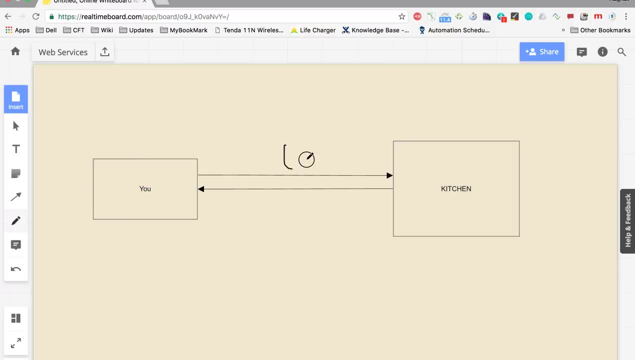 is that person? So that person is a waiter, right? So let us say: this is our waiter who is doing all this communication between you and the kitchen. So this is our waiter, Okay, so his responsibility is he has to take your order. go to the kitchen then make sure the 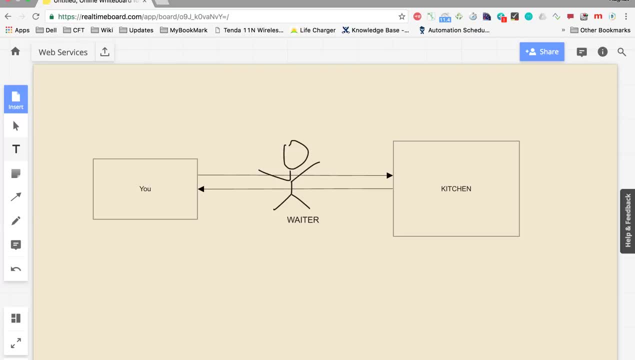 kitchen, Plays the order and serve you back. Now, here our waiter is performing the role of a web service, API, or we can also say web service. He's communicating between two applications and making sure that the communication is proper and successful. Okay, now you might. 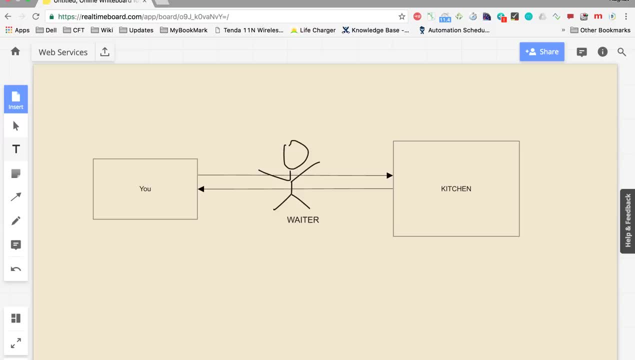 have a question that what is the criticality of the presence of this particular person in this communication process? Even if this person or waiter is not present, you can still go and place your order to the kitchen and then take it from there and have your food. 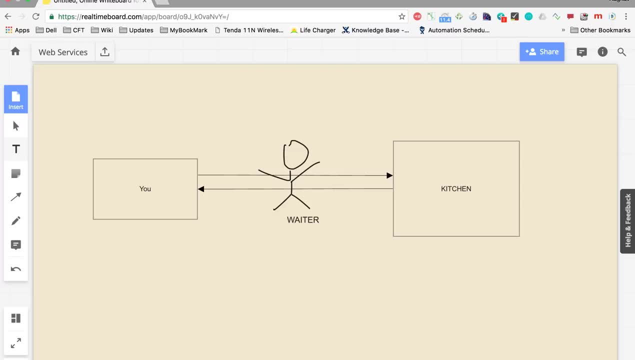 Okay, now think about this scenario: You speak English and the chef who is present inside the kitchen speaks German and you do not understand each other. In that case, here is a whole word: set up person who makes sure that you two applications can communicate with each other, and whatever. 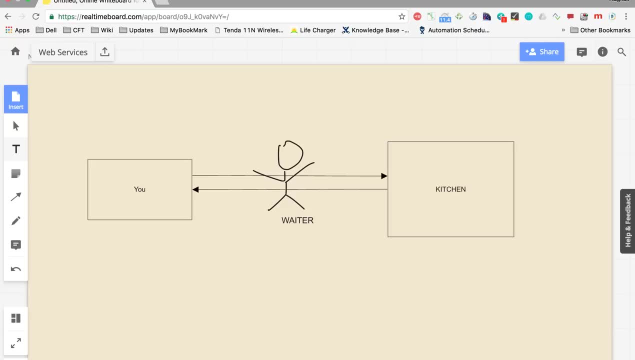 response you have to get from the server, or whatever request a server has to get from a client, is in a format where two entities can understand each other and communicate. So here you are a client and kitchen is a server, and you are communicating with each other. So therefore, the presence of this waiter or web services becomes very important. Let 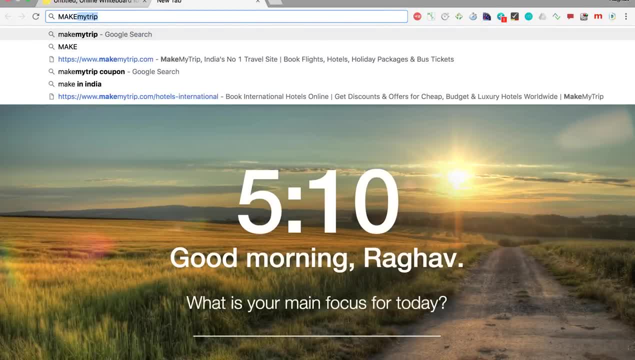 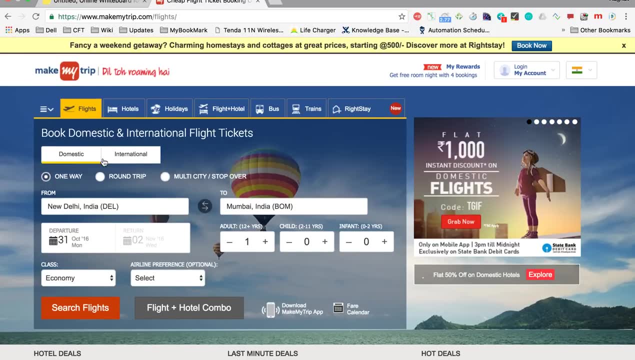 us see a practical example. Let me go to a website like makemytripcom and let us try to book a flight. So I am, I'll, I'm booking a flight from, let's say, India, India, India, India, New Delhi, to Mumbai. Okay, and let me just click search flights So see what this. 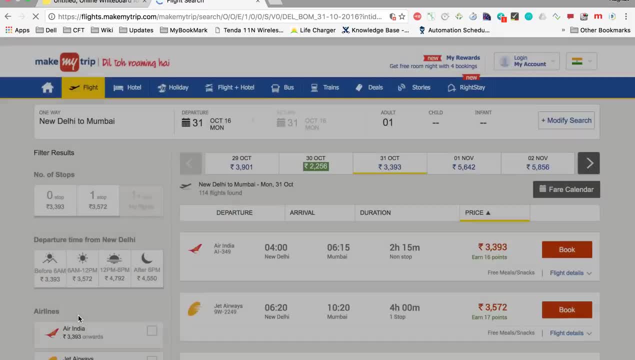 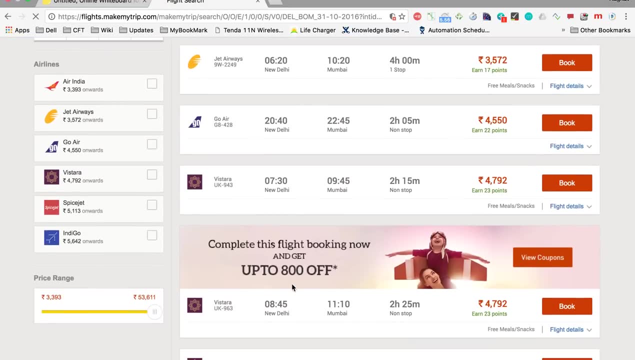 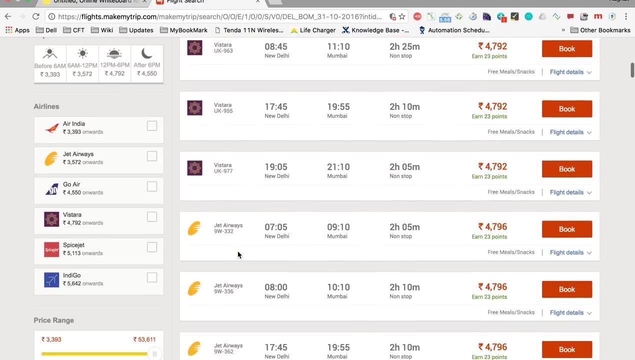 website is doing. It is searching for all the flights between New Delhi to Mumbai on some particular date and within few seconds it has given me all the options. So all the airlines: Air India, Jet Airways, Go, Air Vistara and all other airlines- all the information about. 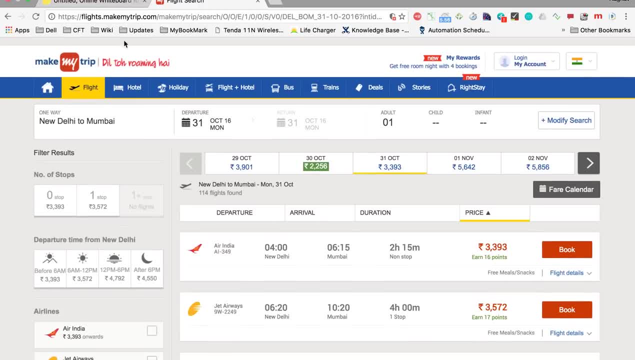 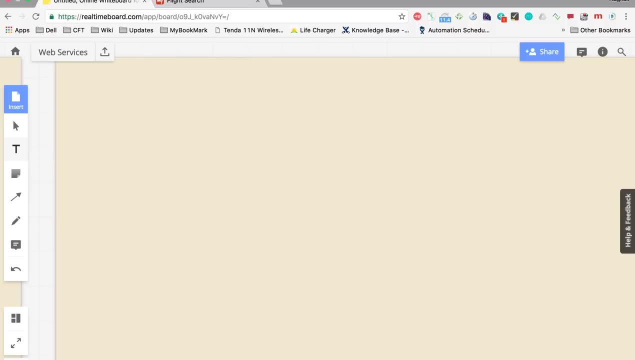 their flights. These have been listed out within few seconds. So what has actually happened here? Let us try to understand this. What has happened here? So let us say: this is the website Make my trip Okay, and this is Air India. Air India. 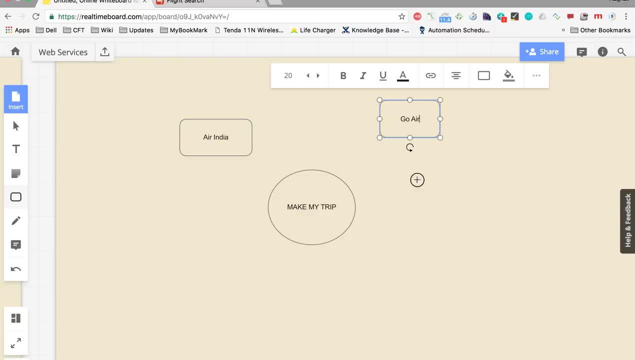 this is Go Air, this is Indigo. then we have Jet Airways and others like Vistara and so on. So what make my trip website has done? in our example? it has communicated between these websites Right. So, whether it is Go Air, whether it is Indigo, it has sent some request to see. 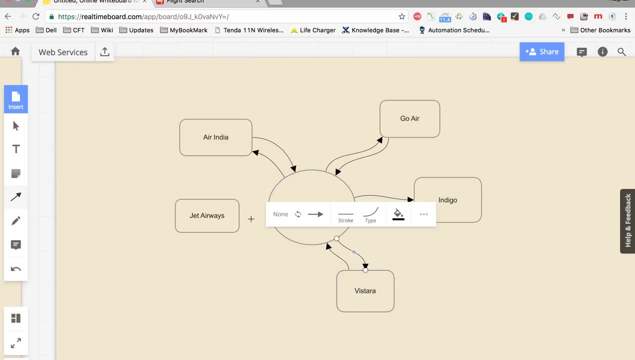 back a response and then displayed the details of all the flights of all these websites. Okay, so this is what has just happened in our practical example. Now, what do you think? How is it possible for a website like make my trip to a QR code? 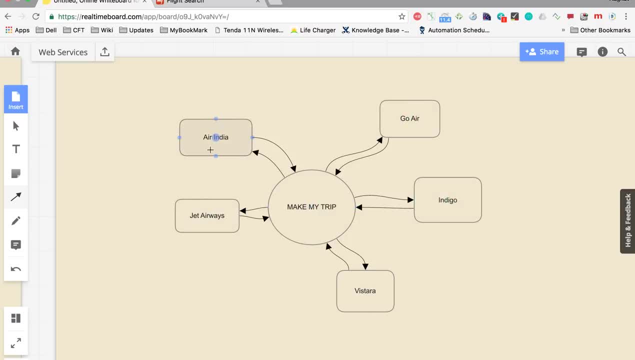 To query the databases of all these websites, all these applications, real time and provide us information of all the flights within a few seconds. Well, one of the ways is: this particular website make my trip, or this particular application has access to the databases of all these websites, of all these airlines. But that might not be the case here, because 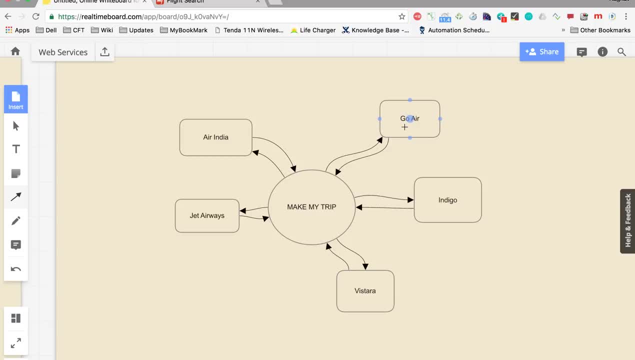 okay, No airlines website or airlines will allow a third party to go inside their database. for some obvious reasons and for some security reasons, it will not allow. So that might not be the case. Okay, they can be a second possibility that these airlines are dumping all the data. 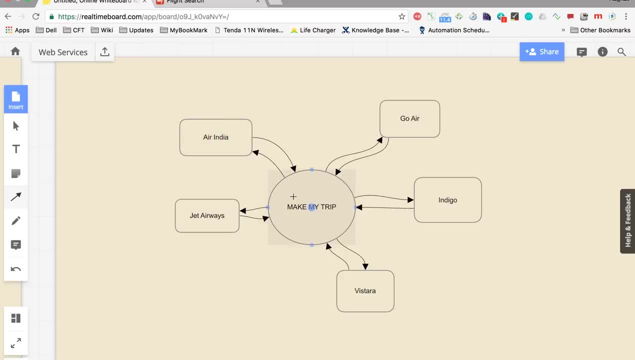 or all the information about their flights, to make my trip every hour or every half an hour. That can be practically possible, But think about the situation. The status of the flights can get changed every second. Okay, in that case we need real time data. What if somebody? 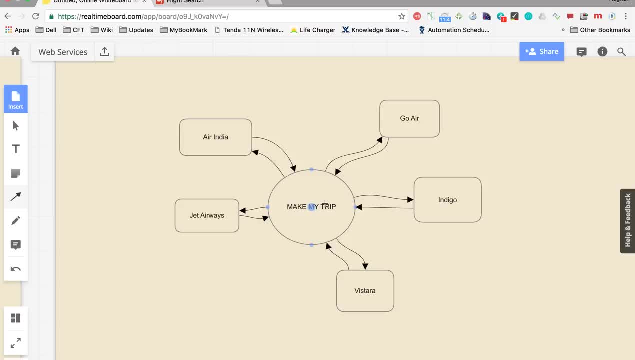 tries to book a flight, but that flight got cancelled 5 minutes ago. but make my trip will show that that is available, and then there will be a lot of chaos, right? So that can- cannot be the case either. Now, what happens here is: 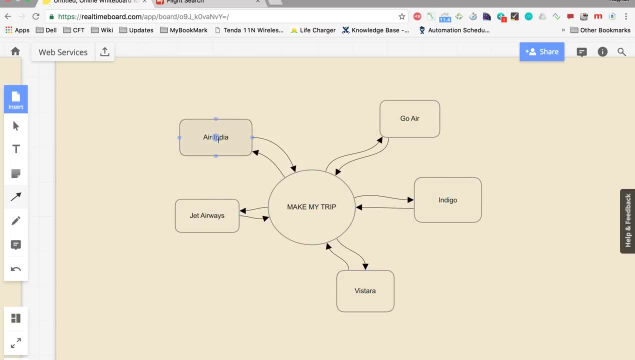 All these airlines have exposed their web services through an API, and this website, MakeMyTripcom, uses those web services to communicate between the airlines. Okay, so it has a common format in which it sends out a request and receives back the response in the same format, and that? 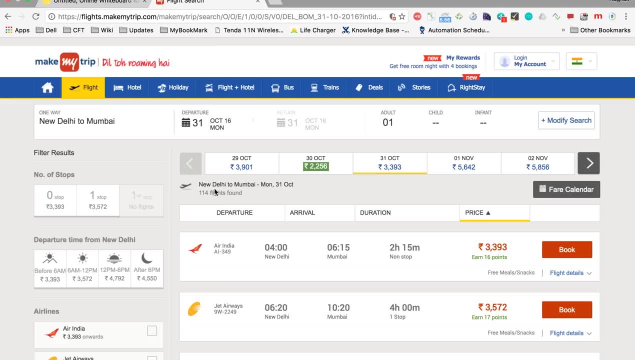 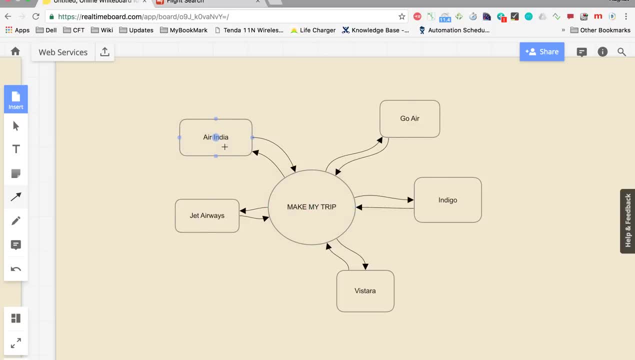 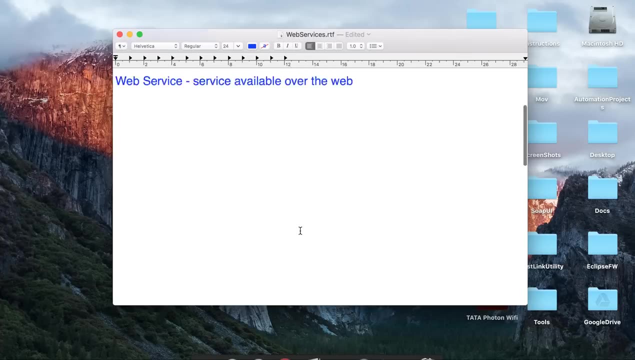 response is shown on their website here. Okay, so this is how they are communicating and this is how they are making use of web services. Okay so now you can appreciate the use of web services. Let me also put this down here. So web services is a service available over.